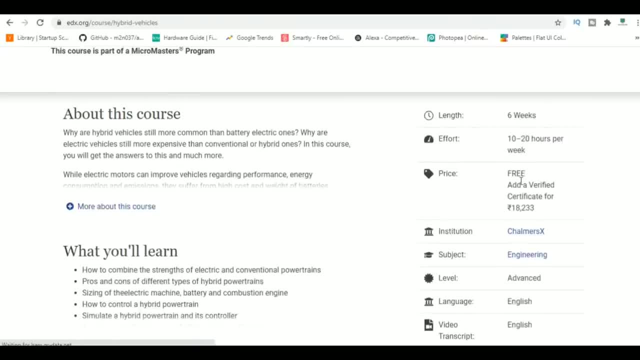 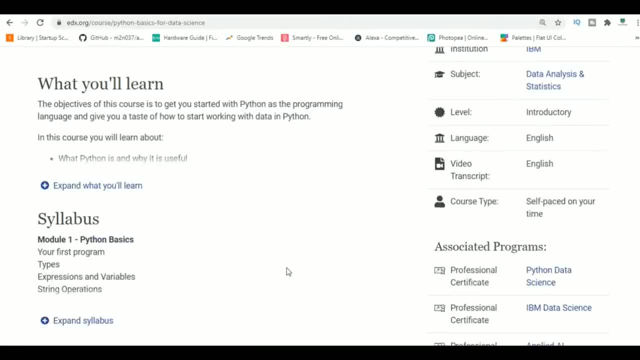 it in your resume. You'll find courses on almost every topic. You can take any course for free, and if you want to get a certification at the end of the course, then it will cost you some money. Other MOOC platforms worth checking out are MIT Online Courses and Coursera. 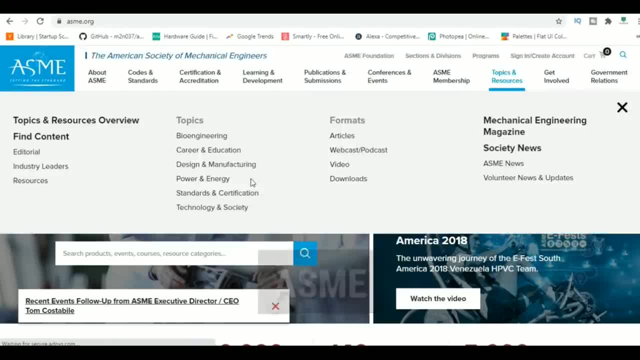 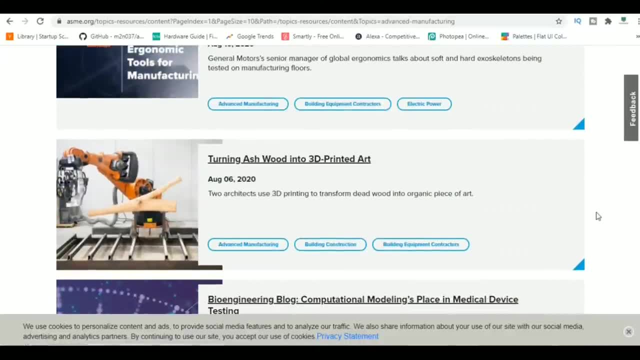 At number 3, we have ASME. ASME, or the American Society of Mechanical Engineers, is a great website to learn industry-standard design codes and principles. To give you an example, you can learn standard design codes for turbo machinery pumps, piping systems, pressure. 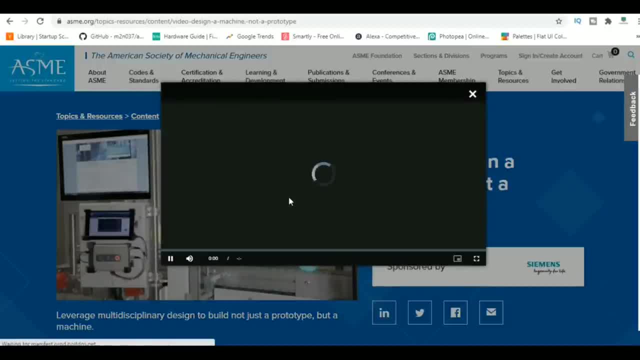 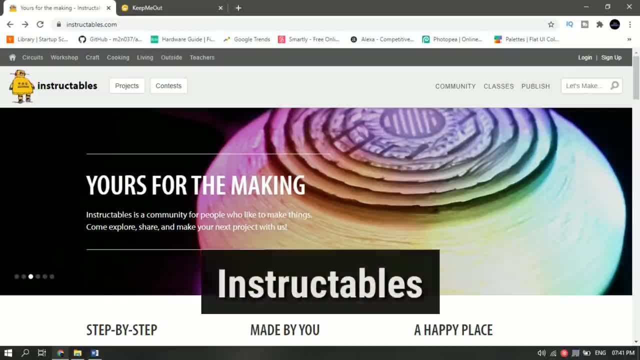 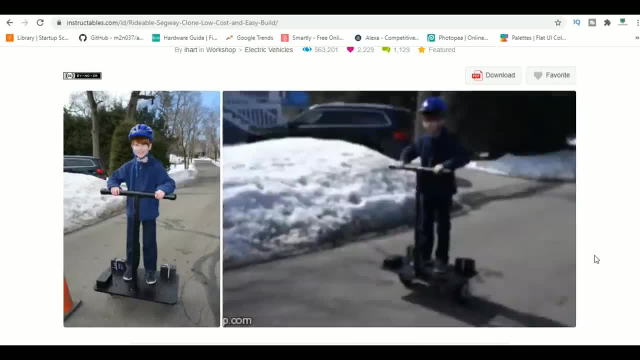 the industry. You'll also get a chance to learn some of the most important things in the industry. At number 4, we have Instructables. Part of being a mechanical engineer is you can design things which we use in real life. Instructable offers easy-to-follow, simple how-to guides. 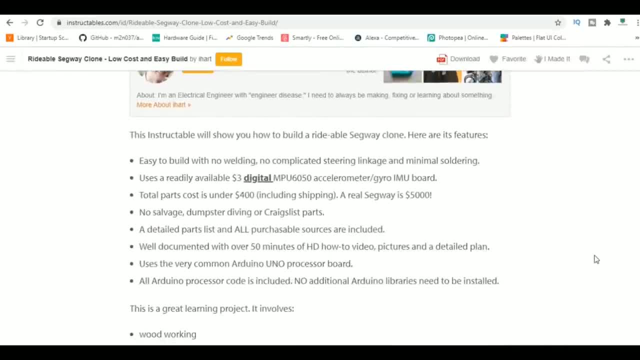 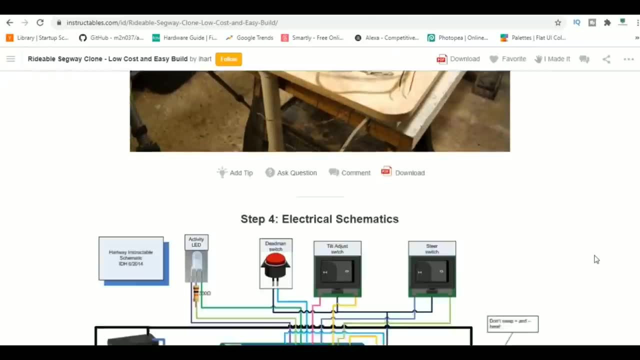 to make cool projects. If you like making things on your own and fixing things yourself, then you should definitely check them out. Some cool projects to name are making a snake game on a breadboard and building a rideable Segway. At number 5, we have идemechanica. 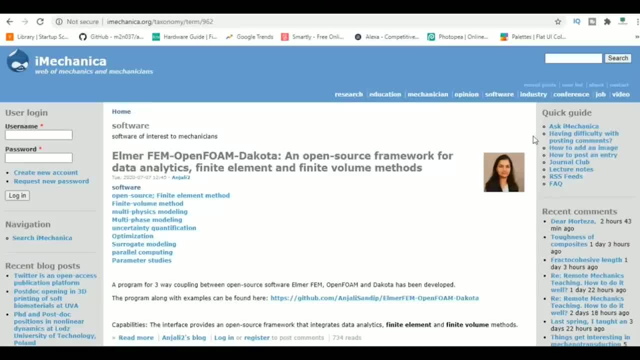 The two hashtags on the artistic board are: imechanica возвращa. moment of creation. There are eight of them all. The most important mook test is the one you click on the box and come up after nothin". Anika is a community of engineers who share their knowledge about various industry standards. 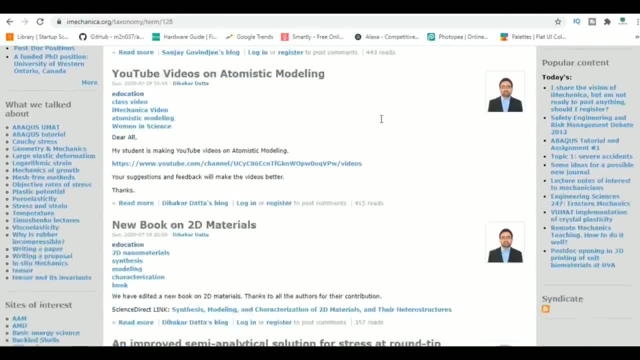 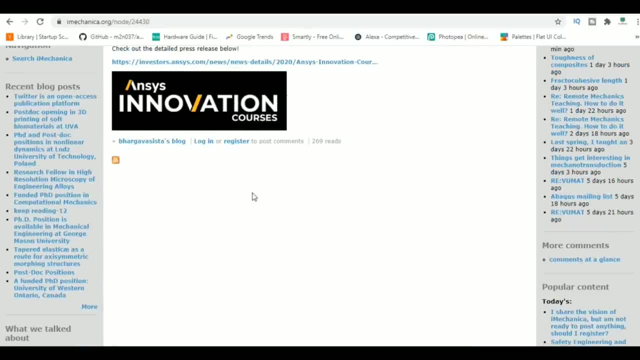 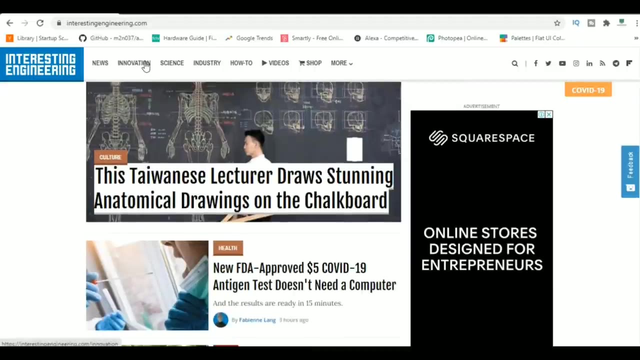 teach a particular software, share their research paper and more. You can learn from industry veterans, researchers who have spent their life in the industry, and learn about a vast variety of topic And website. number 6 is Interesting Engineering. Interesting Engineering is a community of like-minded engineers who share a new idea. 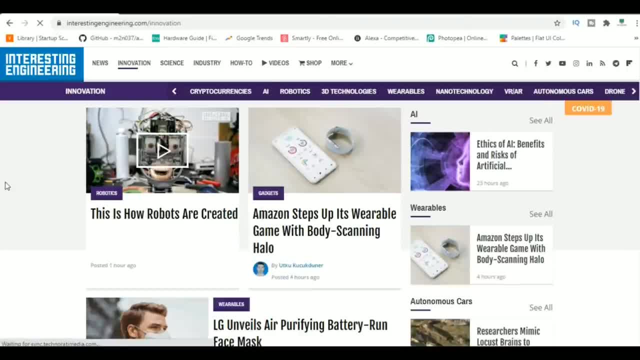 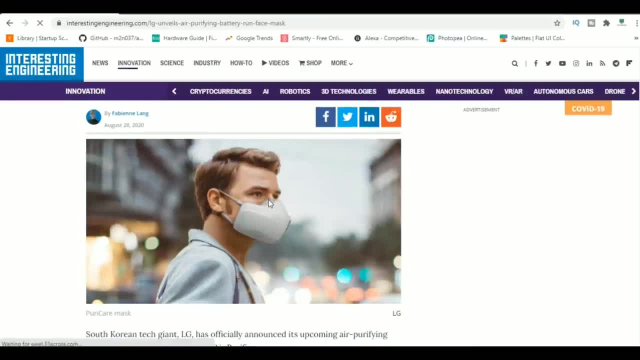 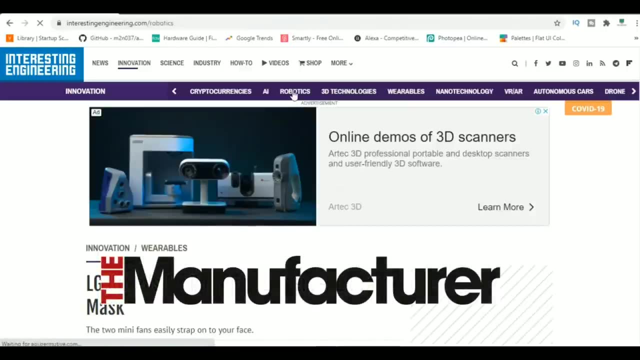 any upcoming technology or an engineering breakthrough, whether it's a device that can charge your mobile in seconds or it's the latest model of Boeing that has launched moments ago, Interesting Engineering will keep you updated with all the new things happening in the industry. Another similar website is TheManufacturercom.